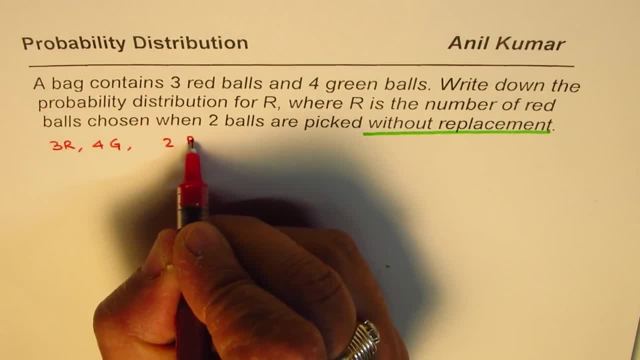 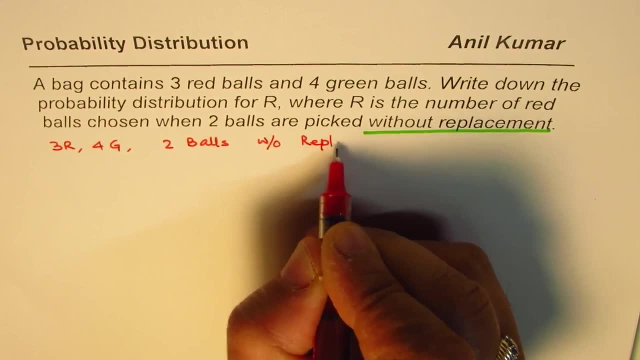 solve such a question. Now, in all, we have seven balls, As you can see, three red balls are chosen when two balls are picked. and we are picking two balls, Two balls are picked without replacement. So that is the key: without replacement. So what happens If? 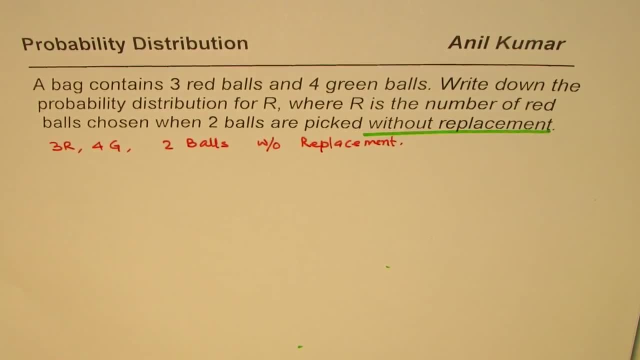 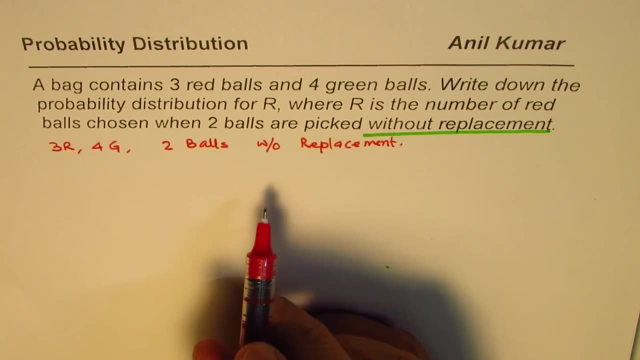 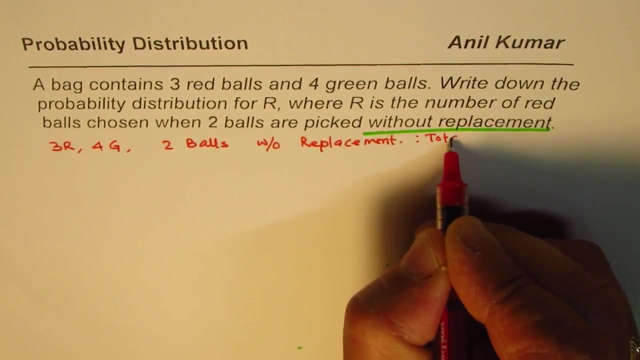 you pick a ball, the number of balls decreases. That's important to understand, Is it okay? Now let us see how to solve such a question. Now, in all we have seven balls, as you can see. So total we have three plus four, which is seven balls, Is it okay? So total there. 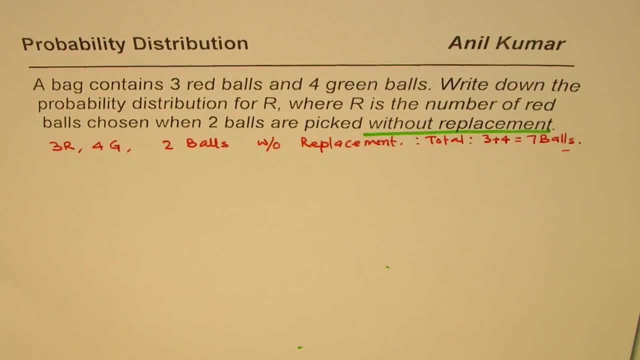 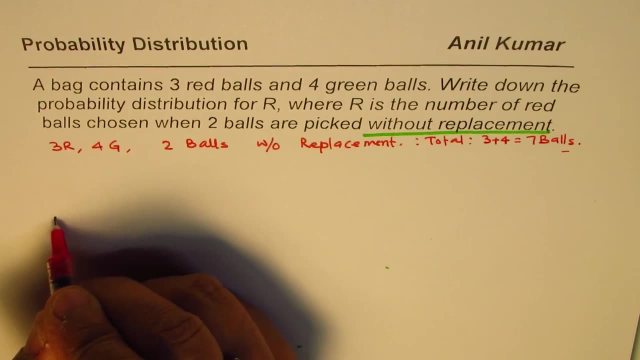 are seven balls. Now. that will help us to find the probability right. So now let's begin by choosing the balls. So when we make the first selection, let's say, let's make it here. So when we make the first selection, we could get either a red ball or a green. 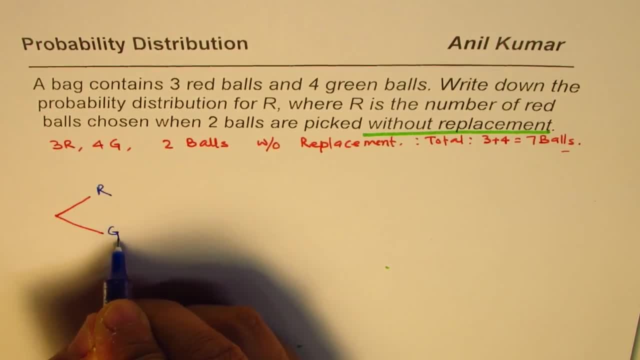 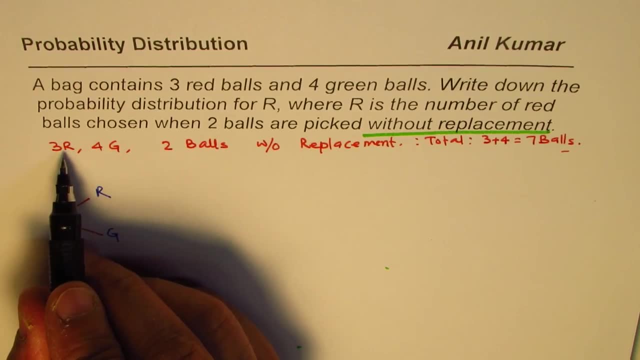 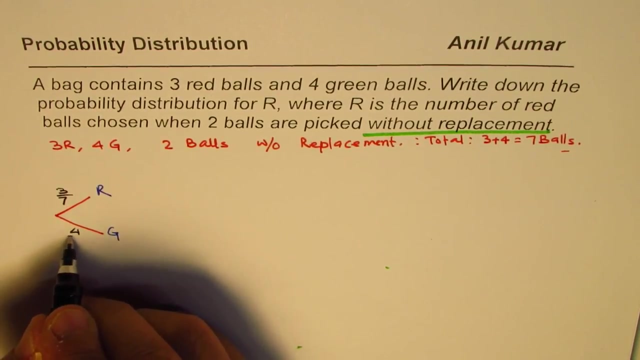 ball. right, So that is the option. So we could get red or green. Now what is the probability of the red ball? Since there are three red balls out of seven, probability of red ball is three out of seven, Is it okay? And four out of seven is for the green ball. Okay, So that? 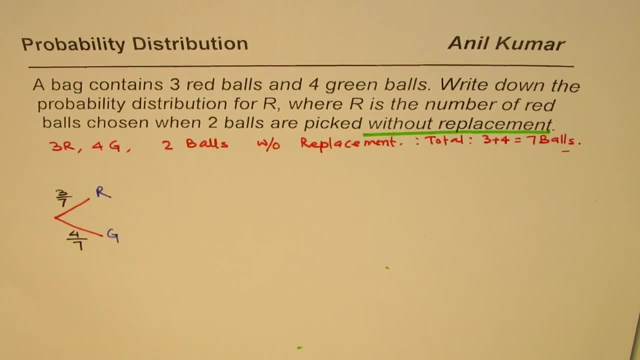 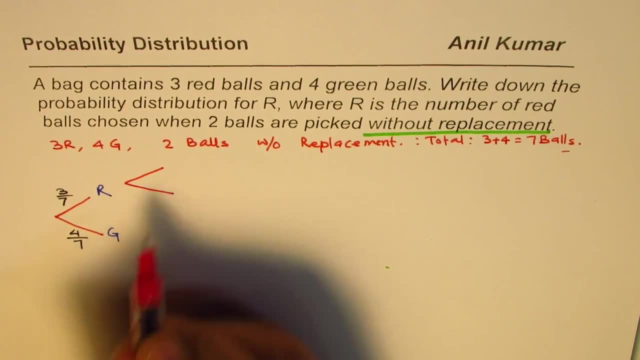 is how first picking is done. And now again, if we pick the second ball, and let us say that the second ball is three out of seven, then in that case what happens Now? well, the probability is you could get either red or green. What is the probability of picking? 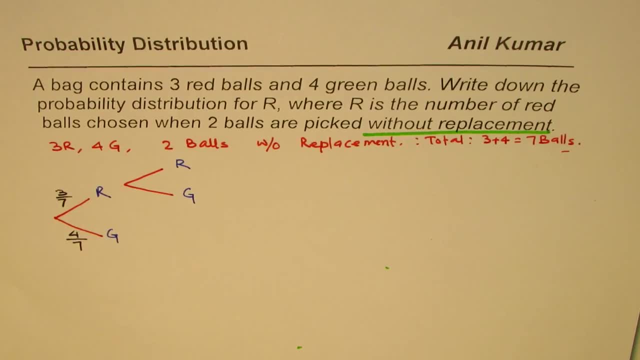 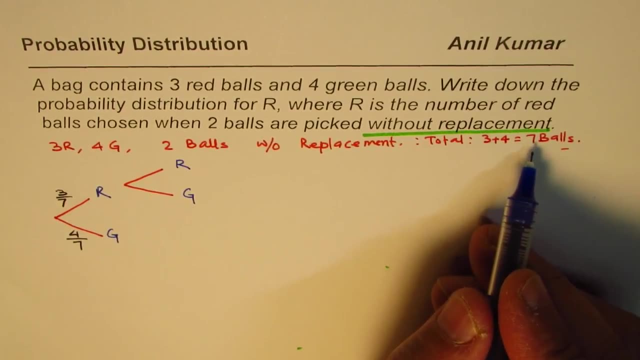 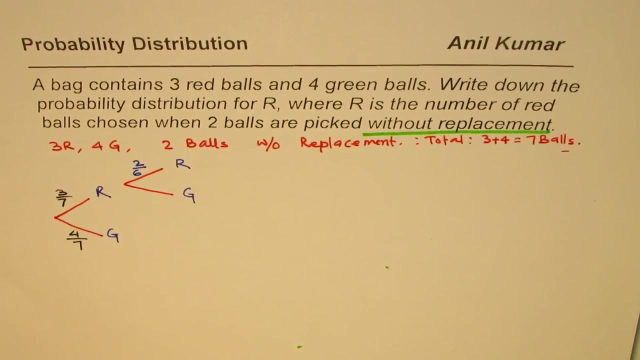 red when we have already picked the red ball. Well, clearly there is one less red ball right And in all out of seven we are left with six right. So two out of six, Is it okay? Does it make sense? So second time, it is two out of six. As for the second time, 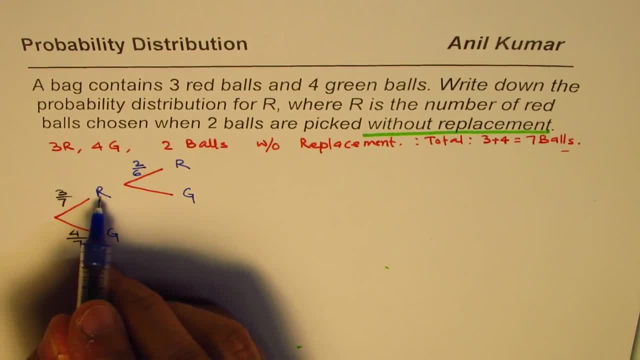 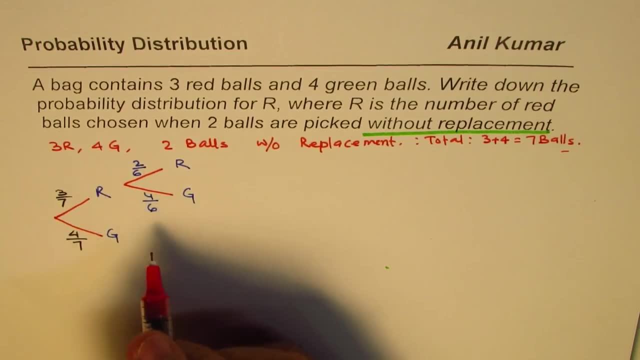 as far as the green balls are concerned, there are still four, since we picked red first. So this is four out of six, right? So that is how we could do Now in the second case, if you have picked green first, then the case could be you could get combination of red. 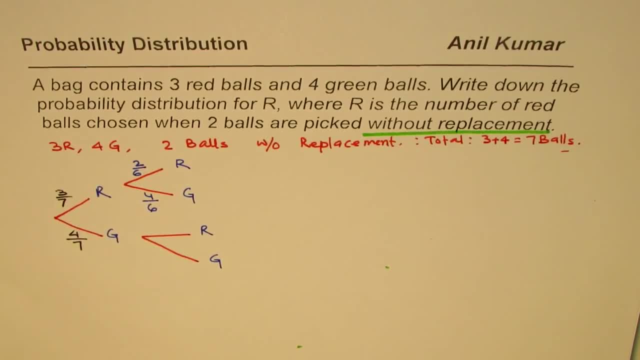 and green, of course, But in this particular case, since we picked green earlier, so we have three red balls right And out of six, So it is three out of six. One ball has been picked right Now, green has been picked earlier, So green number decreases by one. 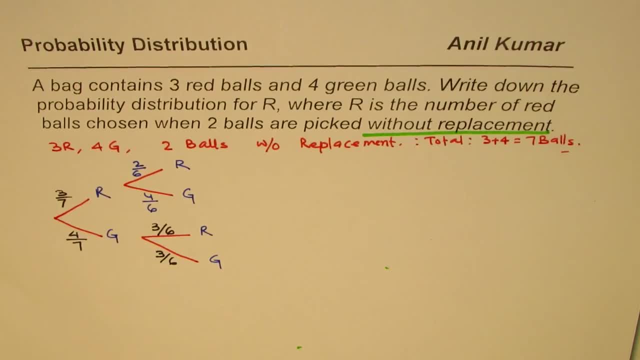 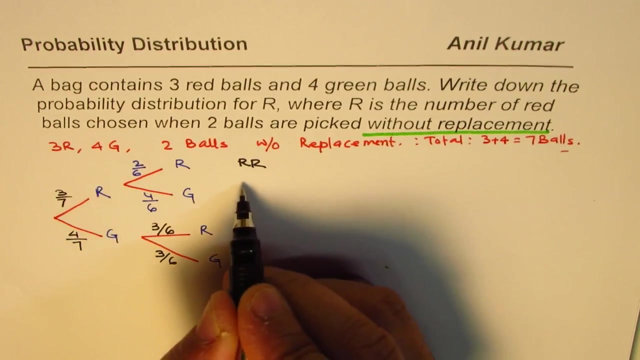 So it becomes three out of six. So that is the tree diagram which actually shows the position. whatever we have right Now here, the combinations are that we have two red balls, So we could have red and green, We could have green and red, Or we could have two green. 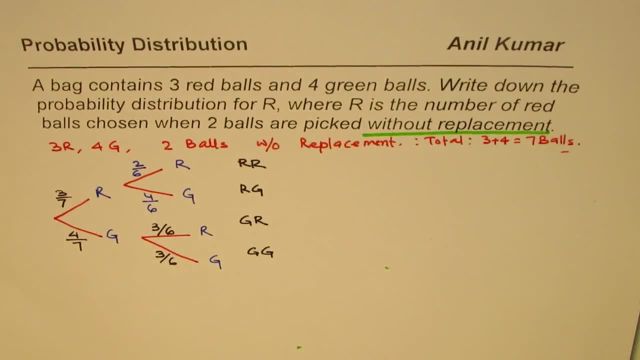 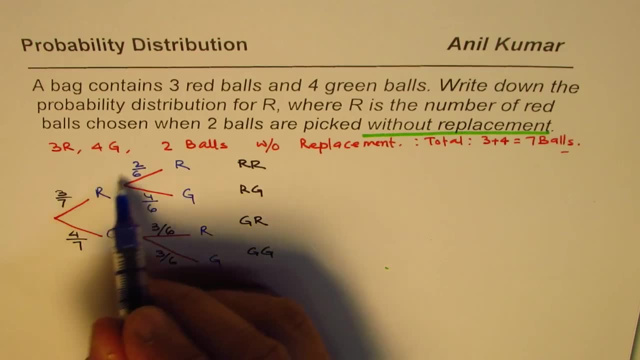 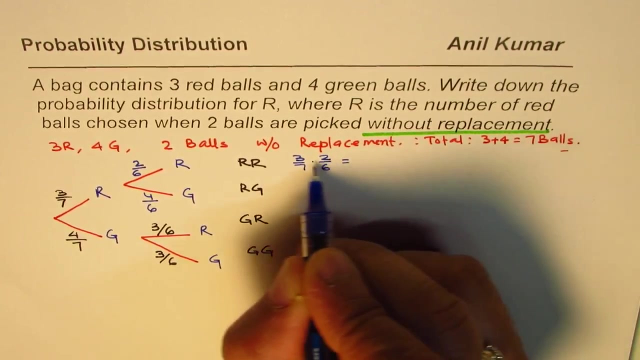 balls. okay, Let us also calculate their probability simultaneously, right? So two red balls, in this case, will multiply these two numbers. So it will be three over seven times two over six, correct? So let me write this as six over forty-two. okay, The second one. 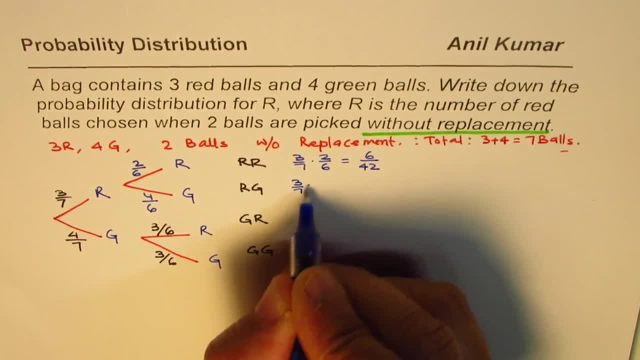 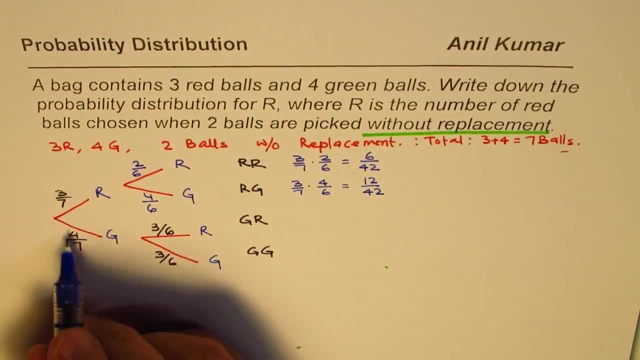 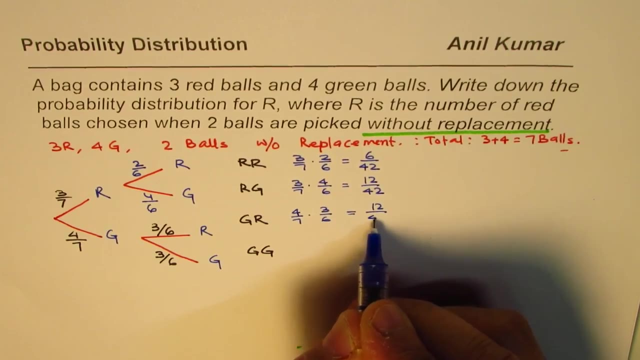 here is three over seven times four over six, That will be twelve over forty-two. And then we have four over seven times three over six, So four times three, twelve over forty-two. And the last one here is four over seven times three over six, which is again four. 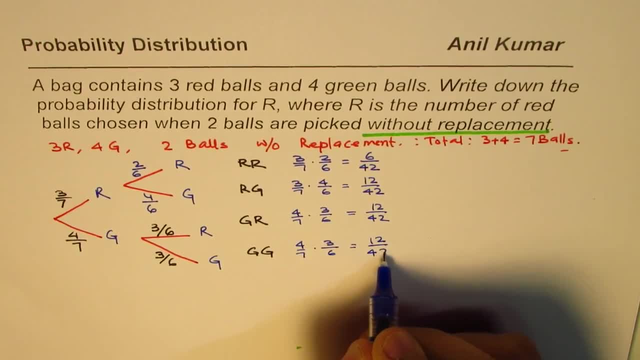 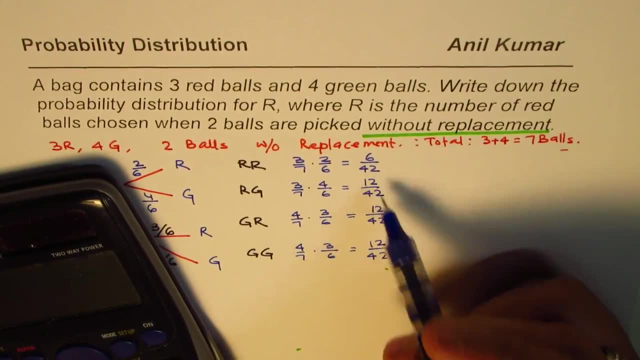 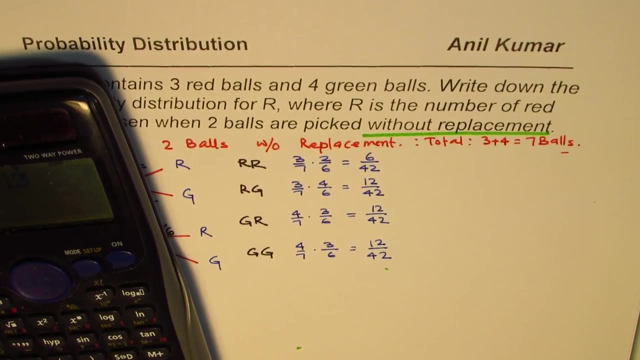 times three, twelve over forty-two, correct? So these are the probabilities. Let us check if it is right, So we can add all these up the numerators. We have six plus twelve plus twelve plus twelve equals to what, Forty-two, right? So that means the answer is correct. 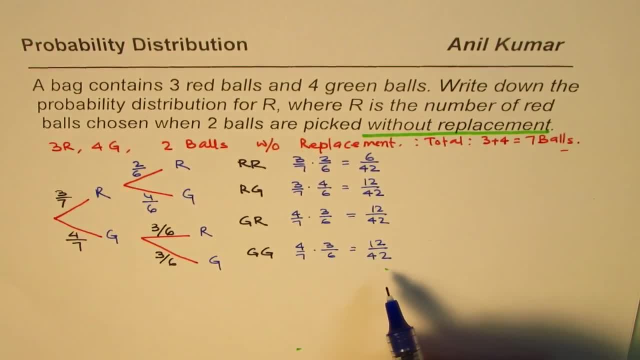 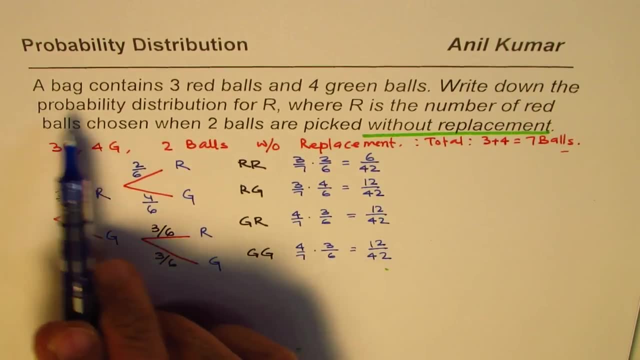 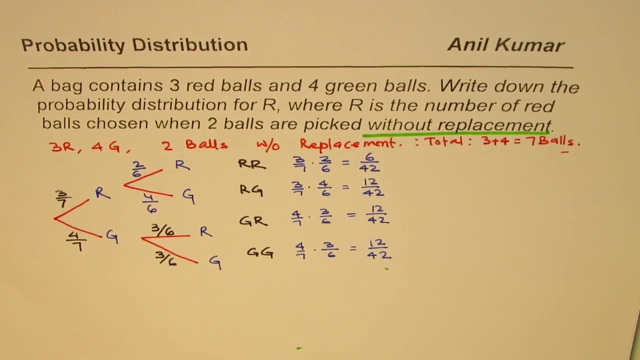 right. So the probability adds up to one. Perfect. Now let us read the question once again. Let us try to understand. what are we looking for. A bag contains three red balls and four green balls. Write down the probability distribution. So we are looking for probability distribution. 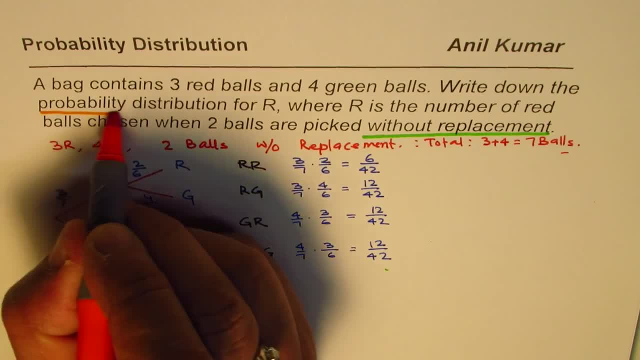 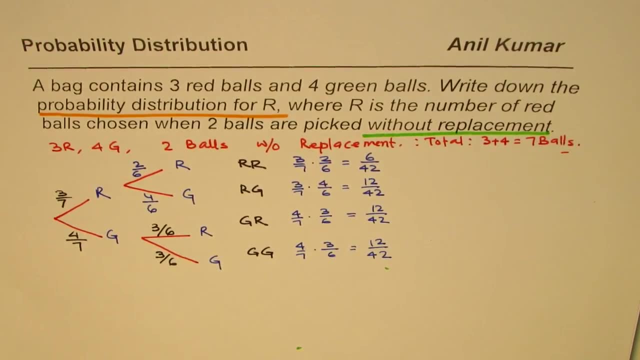 What is that Probability distribution for r, where r is the number of red balls chosen, right? So let us define our random variable, which is r. So let us define. So let us define our random variable: r be the number of red balls, Is it okay? So the 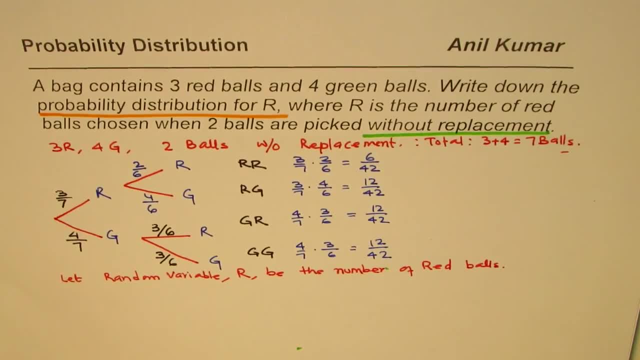 number of red balls is our random variable defined. Now, clearly, when we are having two balls, the possibilities are the following: Two balls would recognize the two of them. One would recognize the two of them, The other would not. How about two'm? enough simply. if we those two are equal to zero. So we have two red balls and another one, but two is zeroax And the other one has two zero's. Now what we have to do is to find the million or thousand times three. overshire double or equals two to zero plus twelve over squelch. 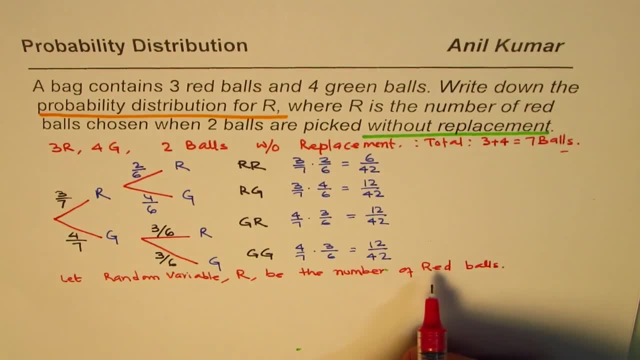 Ok, So three to two equals I, So three to two is number of�じゃない from one to another, So that we could get either no red ball right, or we could get as we have here, or we could get one. 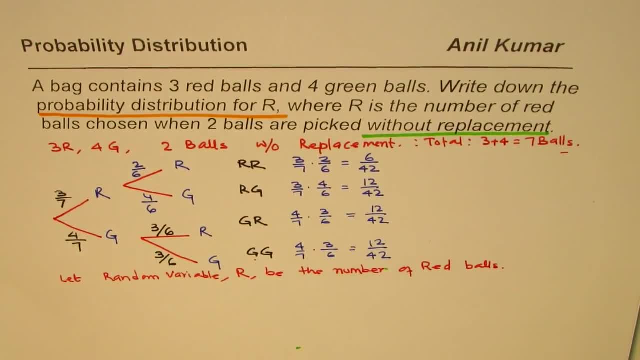 red ball or two red balls, Is that okay? So there are these three possibilities, right? So when we make the distribution table, let me create one here, and then we'll add these probabilities and fill the gaps- Then what are we looking for here? We are looking for the. 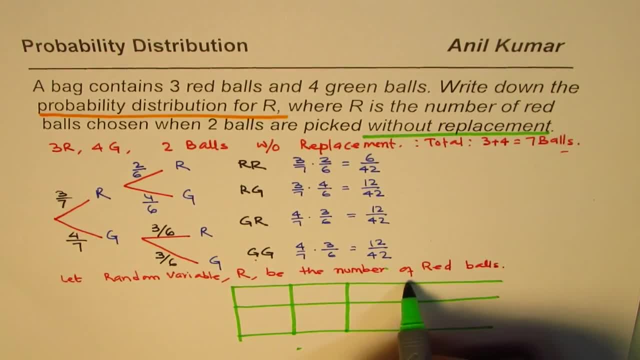 probabilities when we have one red ball. I mean no red ball, one red ball and two red ball. Is that okay? So that is what the distribution table will give us. So in this case, r is a random variable and we're looking for the probability for r equals to, let's say, small r. 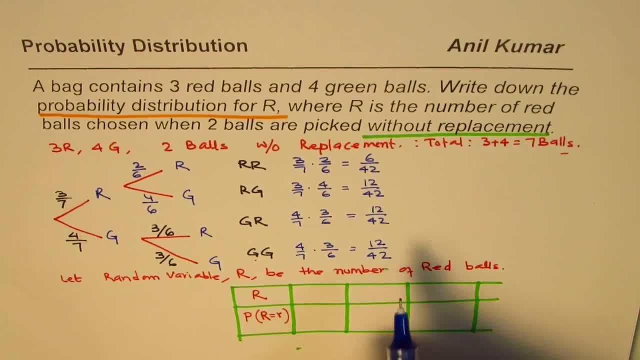 right, And these values- possible values- are either 0,, 1, or 2.. Is that okay? So we're looking for the probabilities. when we have one red ball, I mean no red ball. one red ball Now for 0, that is to say no red ball at all. So no red ball means two green balls, right? 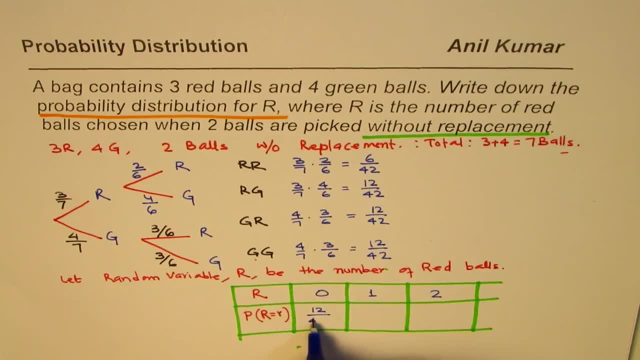 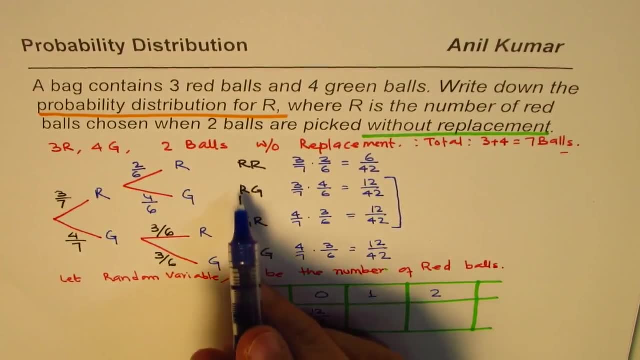 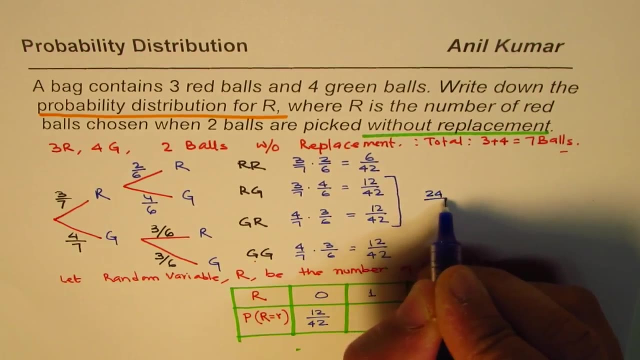 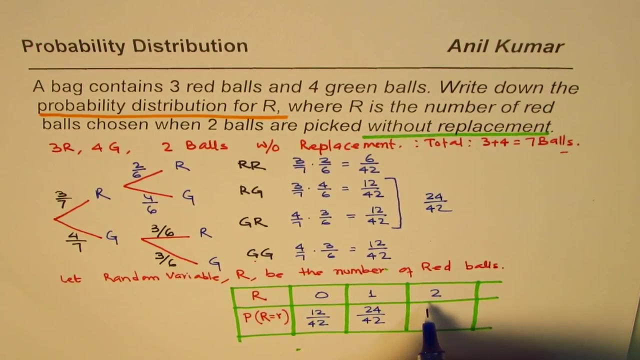 So it is 12 over 42, one red ball. So both these cases actually combine to give one red ball. It could be first red, then green or green and then red, right? So that gives us 24 over 42.. Is it okay Adding these two So we get 24 over 42 and getting both red?